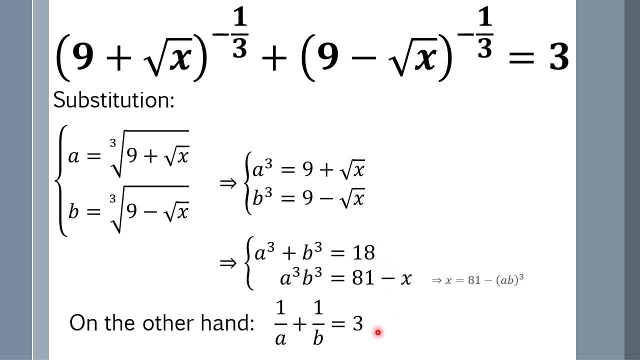 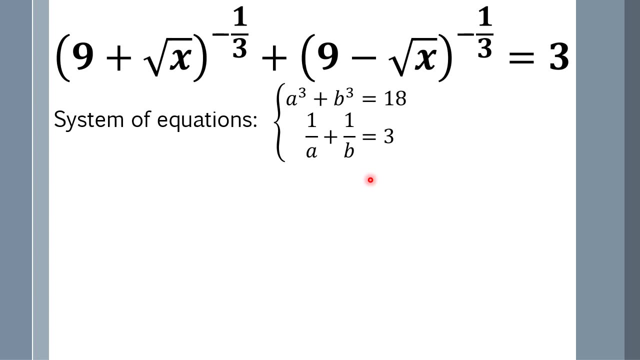 the value of a- b from the other two equations. that means we will get the value of a- b from the other two equations. that means we will get the value of a- b from the other two equations. that means we will get value of x and solve the problem. Let's write down those two equations here. And if we take 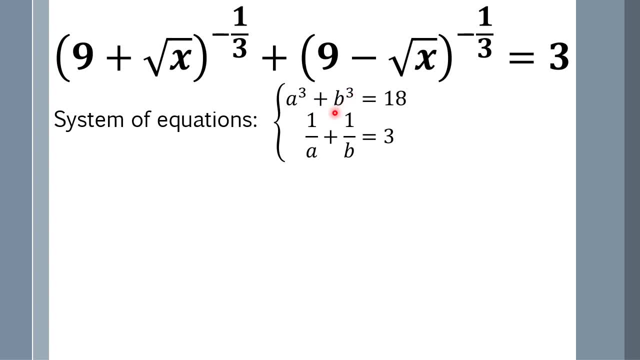 a. look: a cubed plus b cubed and 1 over a plus 1 over b are all the symmetric polynomials, which means if we switch a and b, they are. the expressions are remaining the same. So we can apply the concept of symmetric polynomials here by writing those two expressions as the. 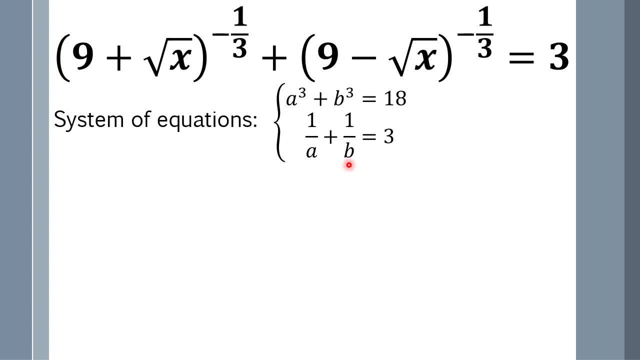 format of a plus b and a times b. To simplify our writing, let's do another substitution here By letting a plus b be m and a times b be n. And a cubed plus b. cubed can be written as a times b. a plus b, times a plus b squared. 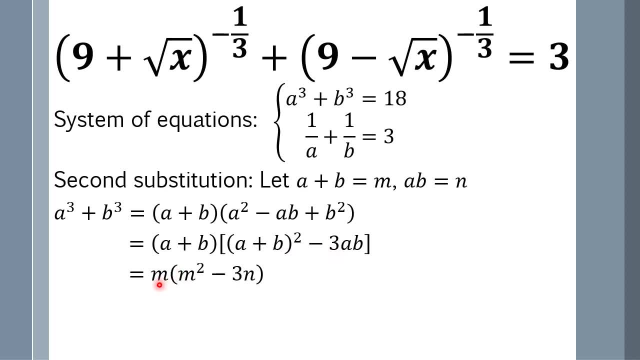 minus 3ab, which is m times m squared minus 3n, And on the other hand, 1 over a plus 1 over b can be written as a plus b over ab, which is mn. So the previous two equations can be written as: m times m squared minus 3n equals 18, and m over n equals 3.. 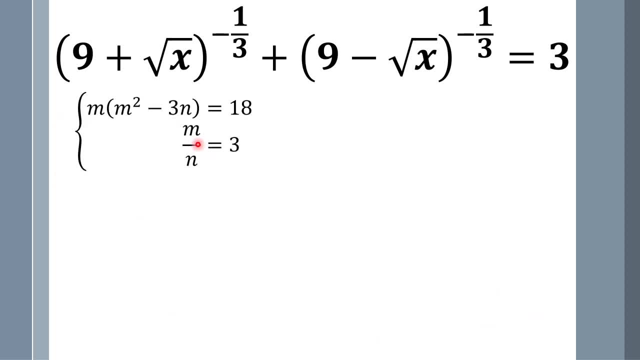 From m over n equals 3,, we have m equals 7.. And this equation can be written as: m plus equals 3n, and we replace 3n with m in the previous equation and get m times m squared minus m equals 18, which is m cubed minus m2 minus 18 equals 0.. This is a cubic equation. 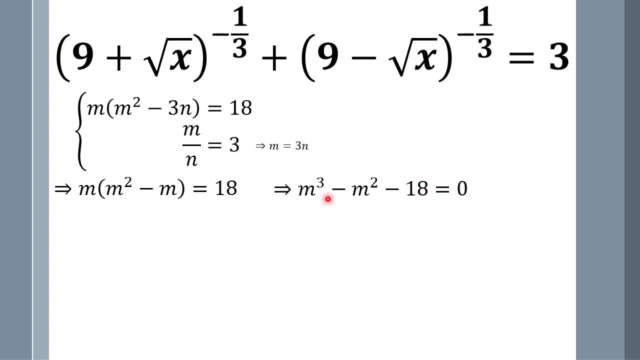 There are different ways to solve this equation. What I'm going to do is to find the factor of the expression. To do so, I write the minus m squared as minus 3m squared, plus 2m squared, and m3, m cubed minus 3m squared can be written as m squared times: m minus 3, and 2m squared. 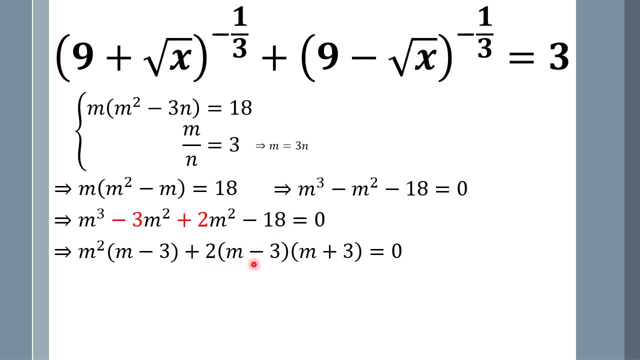 minus 18 can be written as 2 times m minus 3 times m plus 3.. So we can find this common factor, m minus 3. here We put it front and get m minus 3 times m squared plus 2m plus. 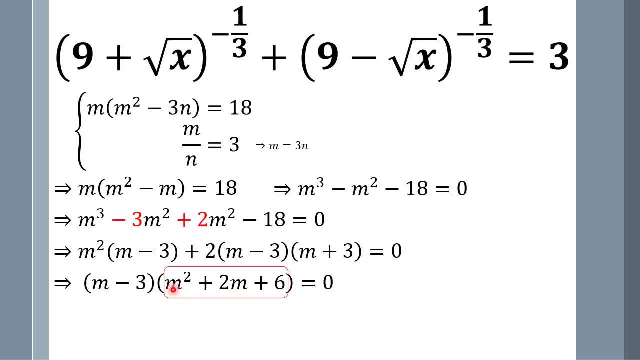 6 equals 0.. For this expression m squared plus 2m plus 6,, the delta value is 2 squared minus 4 times m squared plus 2m squared plus 6.. For this expression m squared plus 2m. 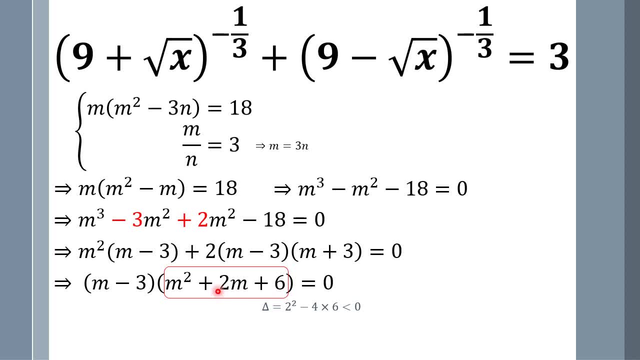 squared plus 4 times m, squared is 2 squared times 6, which is smaller than 0. That means it does not have a real solution. That means the only solution to this cubic equation is m over m equals 3.. And from m equals 3, we can get n equals 1.. And remember, n is a times. 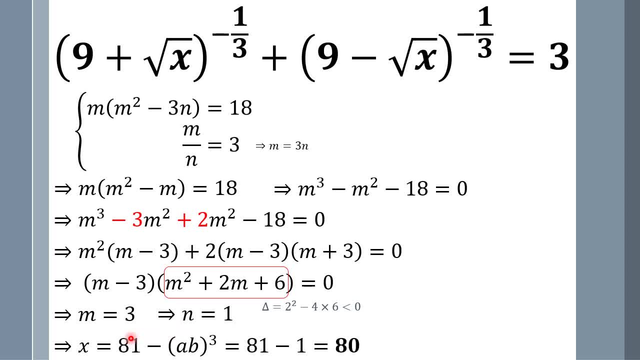 b. That means a times b equals 1.. And finally, x equals 81.. minus AB, cubed equals 81. minus A equals 80.. That's the answer to this question and the problem gets solved. And just bear in mind, you can find out. 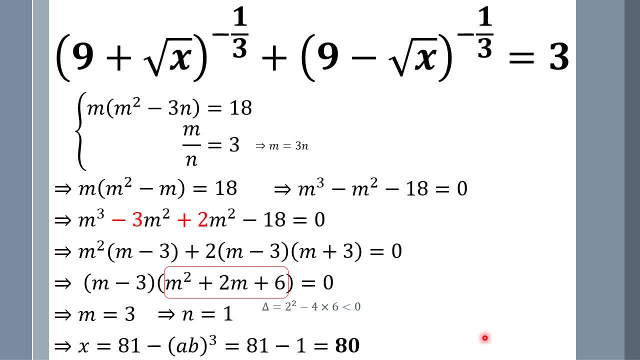 by using the concept of symmetric polynomials, we are able to transfer a question with radicals, cubic rules, square rules to a question without any of the square rules or cubic rules. It will simplify our calculation a lot. The practice. please solve the following equation.